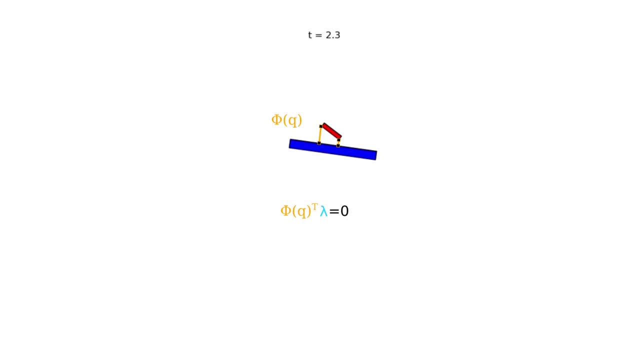 the contact is at the same time between the pancake and the pancake, forces are zero whenever the pancake is not in contact with the pan. In this way, we are able to model contact dynamics, implicitly allowing the non-convex optimizer to solve for the contact forces required by a realistic 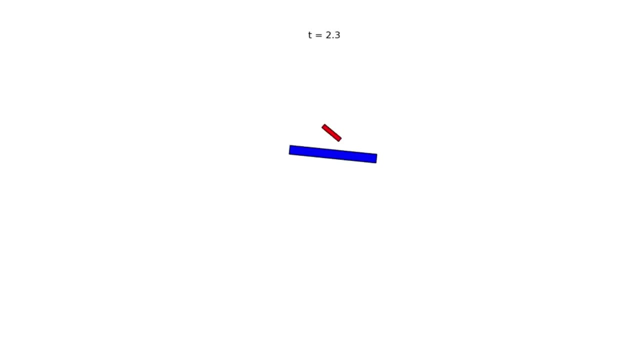 trajectory By employing an implicit model. we do not need to specify a mode sequence a priori, providing the flexibility to make and break contact as needed to accomplish the task. To ensure sufficient accuracy in capturing the system dynamics, we break the total execution time into segments of equal 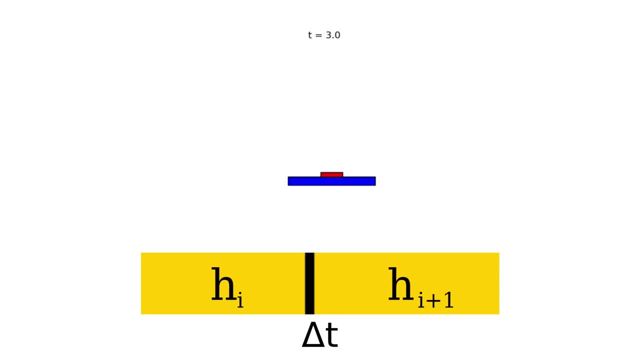 length, then divide each segment into two sub-segments, the duration of which can vary as long as the total length of each pair remains constant. This allows us to use short time steps as needed to model the inelastic collisions between the pancake and pan, while preventing any time steps from vanishing entirely. The 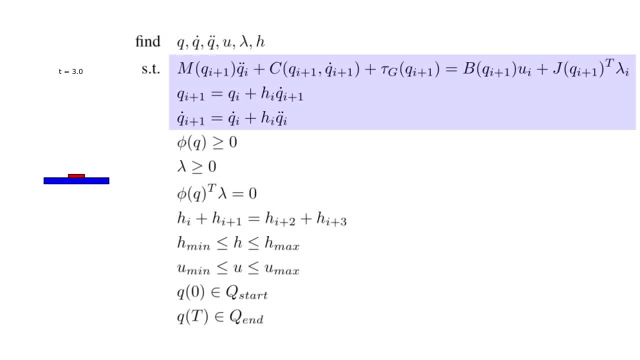 full trajectory optimization problem is shown here. The first three constraints enforce the dynamics of the system, while the next three provide the implicit model of contact dynamics. These two constraints on H allow for variable discrete time stepping, and we also constrain the minimum and maximum. 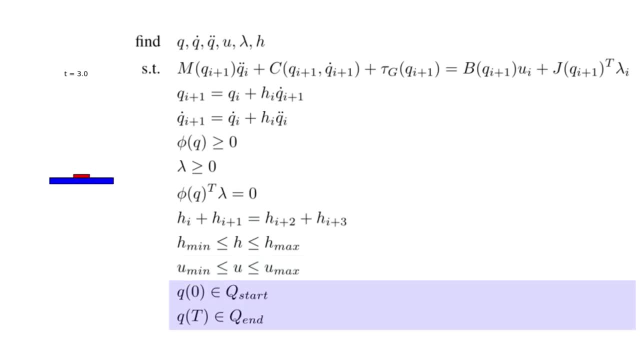 allowable control effort: U. Finally, we also constrain the desired start and end configurations of the pan and pancake. In the example of flipping the pancake, the pancake is initially rotated 180 degrees relative to its desired end configuration. Because we do not need to specify a mode sequence ahead of time, we 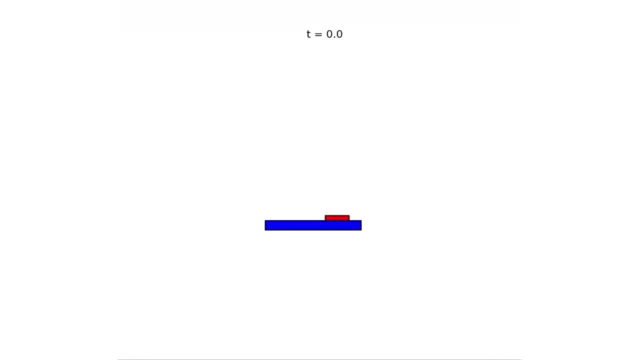 can discover new behaviors simply by changing the start condition. For example, when the pancake starts right-side up relative to the desired end state, we find a trajectory that slides rather than tosses the pancake to the goal position, Although the full system is under. 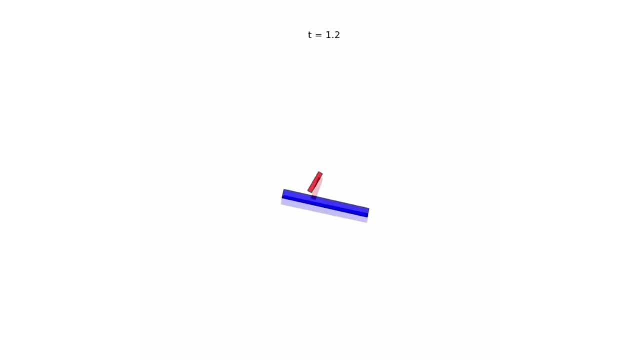 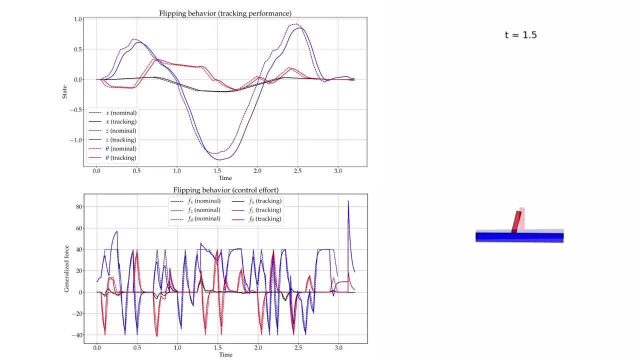 actuated. we can apply partial feedback linearization to the fully actuated pan subsystem to effectively stabilize the multi-contact pancake flipping trajectory without demanding control inputs much in excess of the nominal controls found via trajectory optimization. Solving the inverse kinematics allows us to execute 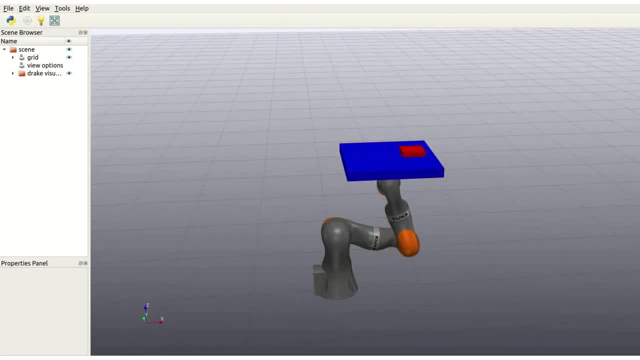 these trajectories on a simulated 7 degree of freedom robot arm.